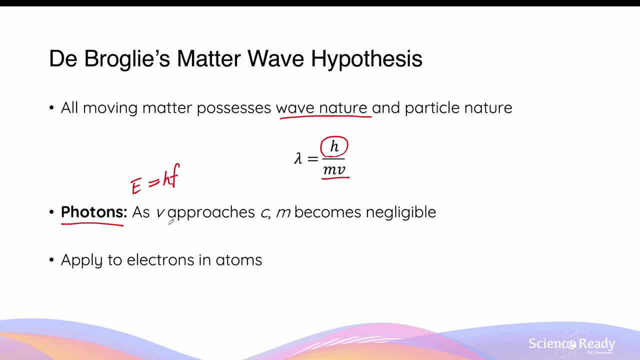 multiplied by the frequency of light. The massless property of photons can be accounted for by de Broglie's equation, as the mass of photons becomes negligible and tends towards zero when the particle's velocity approaches the speed of light, which is c. When de Broglie made this hypothesis regarding matter wave. 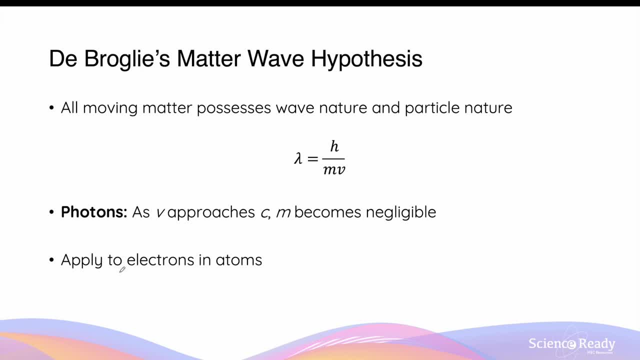 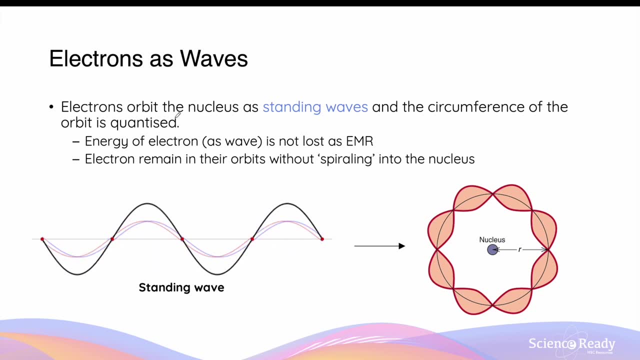 duality. he also applied the concept of matter waves to electrons in atoms, and this will be the focus of this video. De Broglie stated that electrons orbit the nucleus as standing waves And that the circumference of the electronic orbits is quantized, A standing wave is formed. 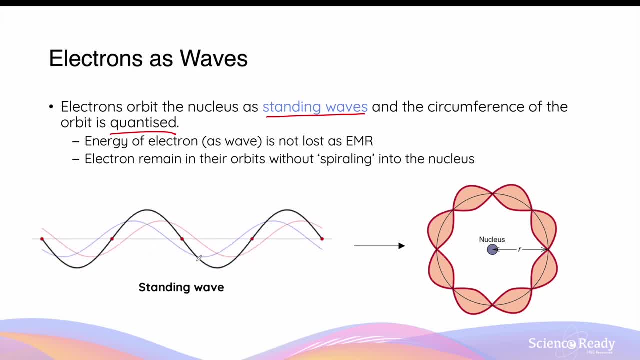 when two waves of equal amplitude and frequency are propagating in the opposite direction shown by the blue and red waves. When they propagate in such a direction, they will interfere in such a way to produce a wave that only oscillates on the spot, and this is shown. 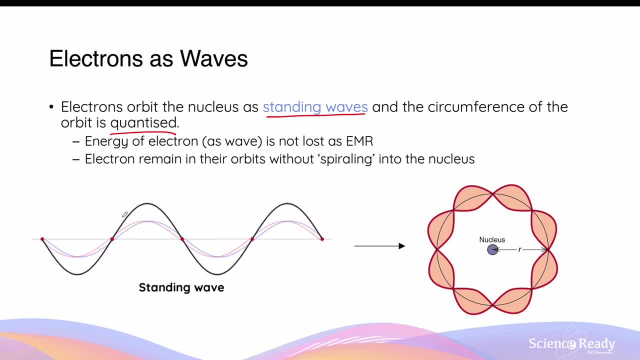 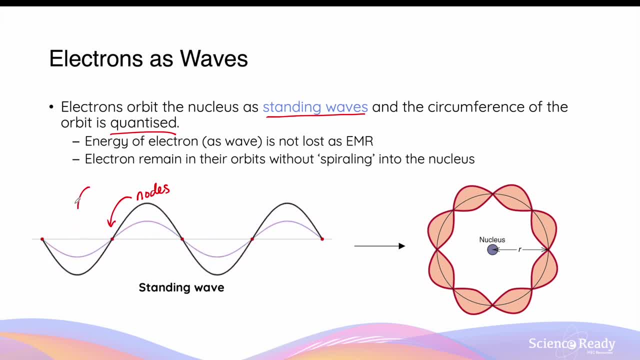 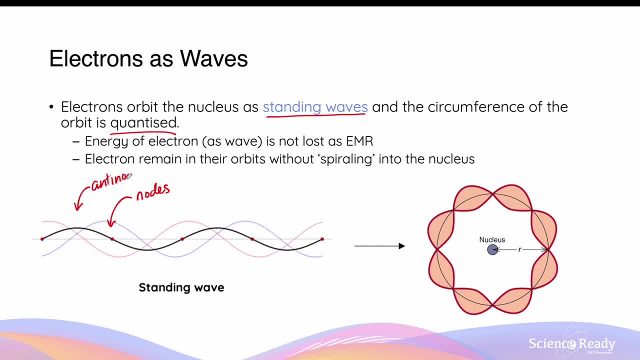 amplitudes occur. these are known as the antinodes of the standing wave. De Broglie explained that atomic electrons should be understood as standing waves around the orbit rather than as particles. So imagine that the black standing wave wraps around the circular orbit that was described by Niels Bohr in his atomic model. In order for a standing 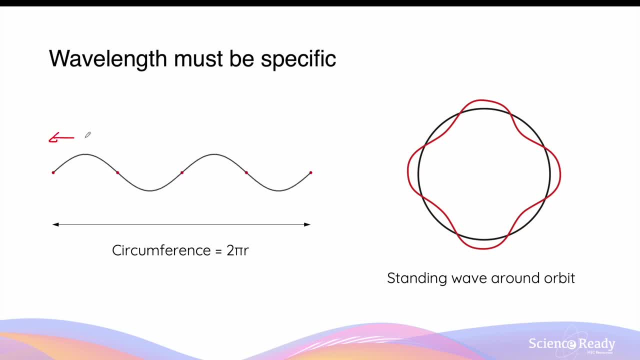 wave to be formed around an electronic orbit. the wavelength of an electron must be specific, such that an integral multiple of the wavelength can fit inside the circumference of the orbit. The word integral means a whole number multiple of the wavelength, So this can be 1 lambda. 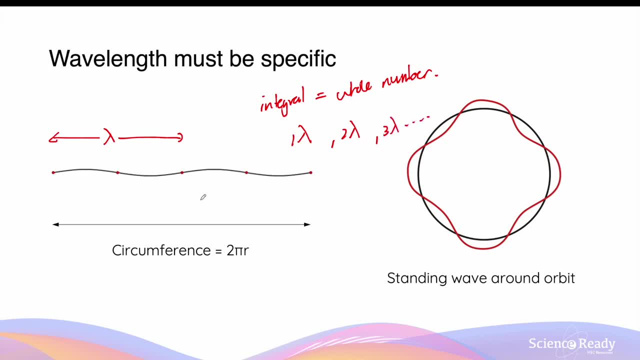 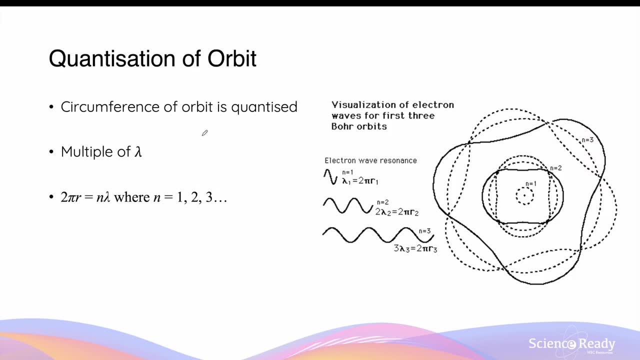 2 lambda, 3 lambda and so on. In this diagram we have exactly two multiples of wavelength, that's being fitted inside the circumference of the orbit. This requirement explains the quantization of energy of electronic orbits, previously postulated by Bohr in his atomic model. The quantized nature of an orbit, in simpler words. 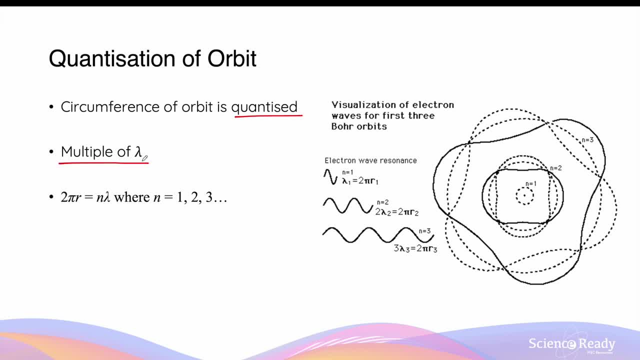 means that its circumference must be an integral multiple of the wavelength of the electron, as we previously explained. Specifically, the circumference of the orbit given by the expression of 2 pi r, where r is the radius of the orbit, is equal to n times the lambda. 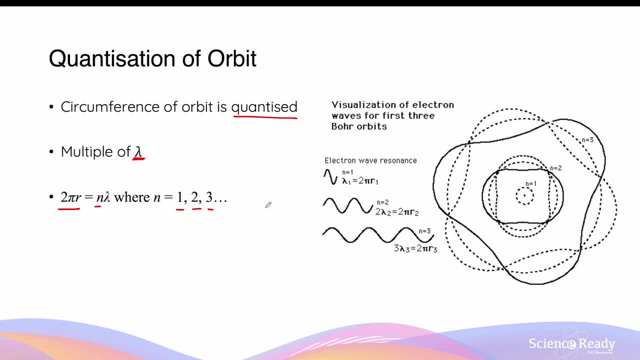 Where n is the integer 1,, 2,, 3 and so on. Here n also corresponds to the energy state outlined in Bohr's model. n equals 1 corresponds to the first orbit, where the circumference of the first orbit, so 2 pi r1, equals to exactly one multiple of the wavelength of the electron. 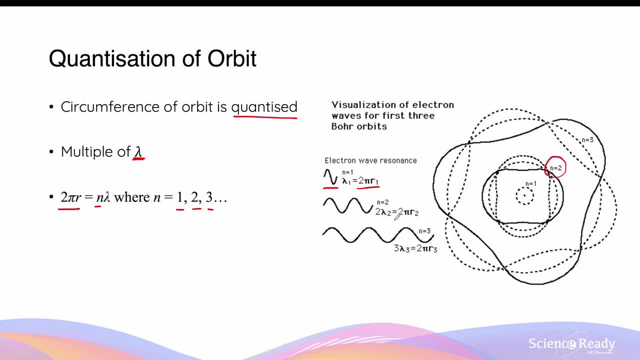 The second orbit corresponds to n value of 2.. This means 2 pi r2 is equal to two multiples of the wavelength. And finally, the third orbit, which corresponds to a value of n equals 3, is a multiple of 3 of the wavelength of the electron. 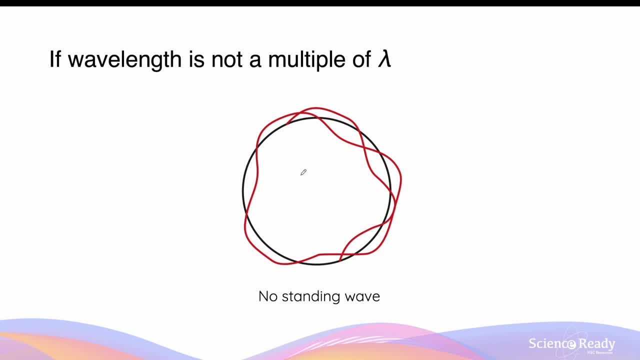 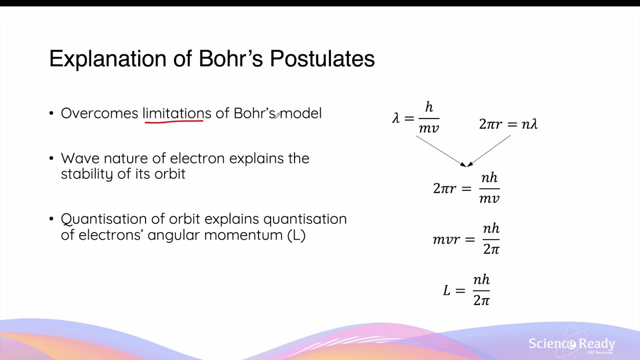 It's important for there to be an integral multiple of a wavelength in the orbit, because otherwise the interference of the electron waves will not result in a standing wave such as what's shown by this diagram. The Broglie's matter wave hypothesis overcomes the limitations of the Bohr atomic model. 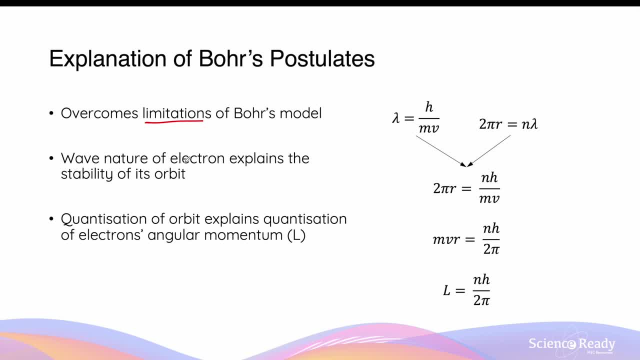 Firstly, the wave nature of electrons as standing waves explains the stability of its orbits. When electrons orbit the nucleus as a wave, they do not lose energy in the form of radiation and therefore they are able to maintain their orbit without spiralling into the nucleus. 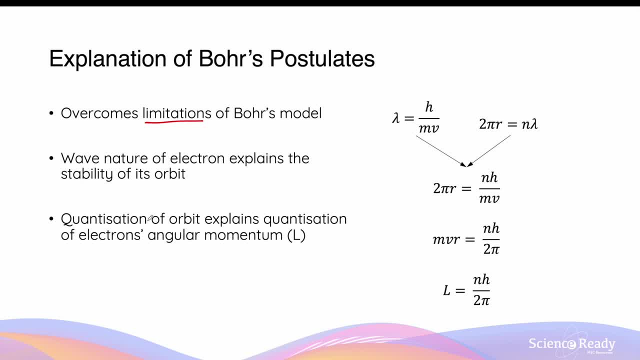 Secondly, the Broglie's equations explain the quantisation of electrons, angular momentum, which was the third postulate of Bohr's model. If we combine the Broglie's equation with the quantisation of the circumference of the orbits, So if we substitute the wavelength with the circumference of the orbits, we get the following: 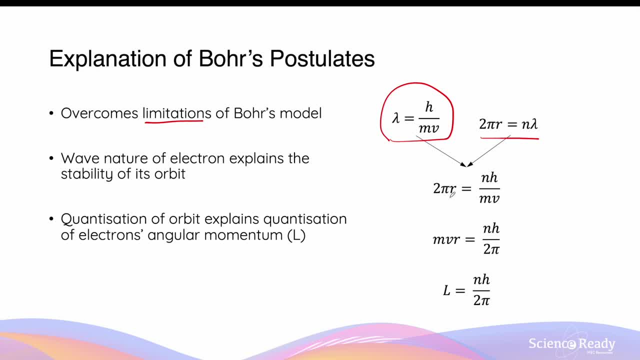 equations. When we multiply mv on both sides and divide 2pi on both sides, we'll get mvr equals to nh over 2pi. We know that mv is the momentum of a particle, mvr is the expression for the angular momentum. 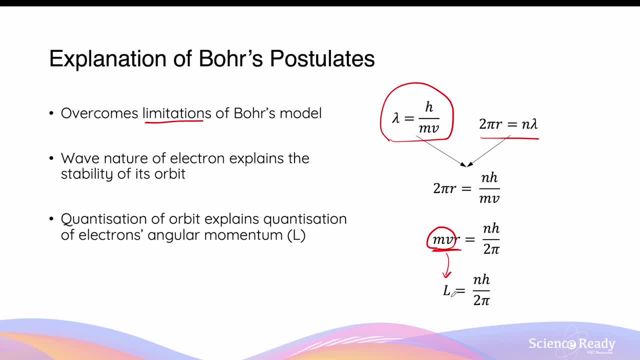 of the electron, which is also sometimes written as capital, L. So the angular momentum in this equation is equal to n, which is an integer, so n can be 1,, 2 or 3 and so on, times by h, which is Planck's constant, divided by 2pi, which 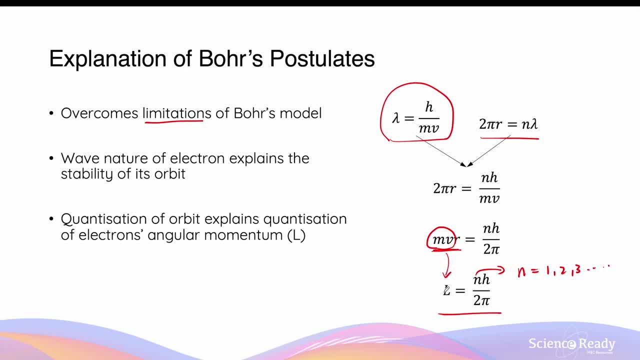 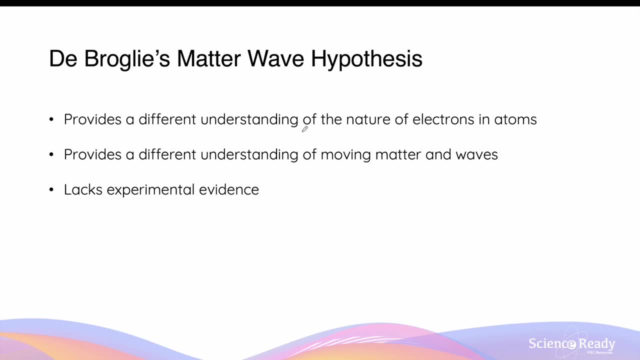 is also a constant. This expression explains that the angular momentum of the electron is a multiple of Planck's constant, divided by 2 times pi. So therefore it supports Bohr's third postulate in his model of the atom. In summary, the Broglie's matter wave hypothesis provides a different understanding of the 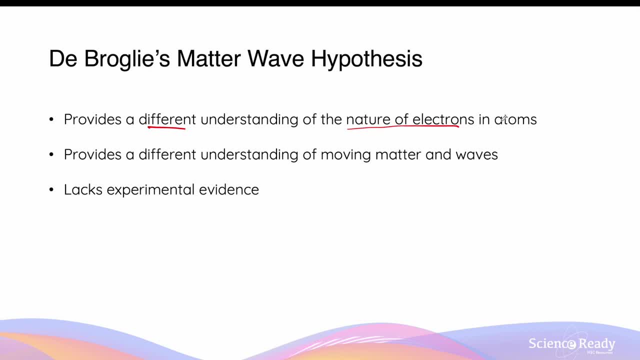 nature of electrons in atoms And, more broadly speaking, it also provides a different understanding of moving matter and waves in general, not just electrons. While this hypothesis at the time accounted for the limitations of Bohr's model, it lacked scientific and experimental evidence. 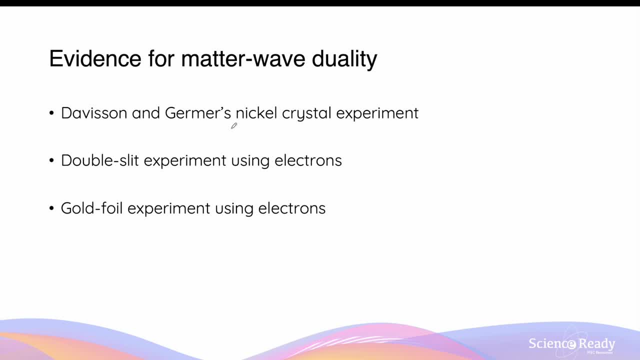 There are three main pieces of evidence supporting the Broglie's matter wave duality theory. The first is Davisson-Germann's nickel crystal experiment. Second is the double slit experiment using electrons. And third is the Goldford experiment. And third is the Goldford experiment using electrons. 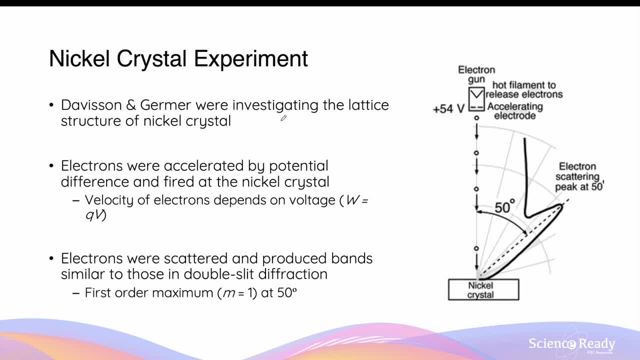 And third is the Goldford experiment using electrons. The nickel crystal experiment took place after the Broglie's matter wave hypothesis. Davisson and Germann were using electrons to investigate the lattice structure of nickel crystal. In this experiment, electrons were accelerated by a potential difference and further fired. 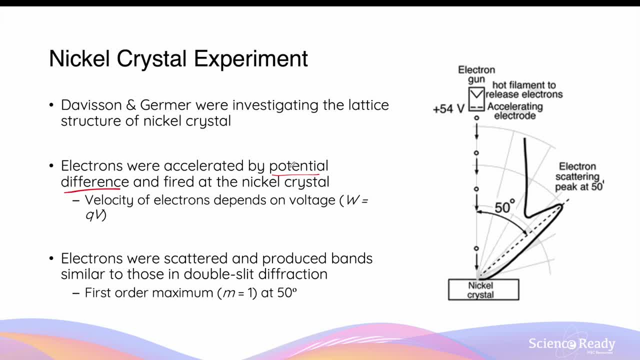 at the nickel crystal that was to be investigated. In this case, the potential difference did work on the electrons- according to work equals q times pi V- And as a result, the work done was straightforward: The electron was transformed into the kinetic energy of the electrons. 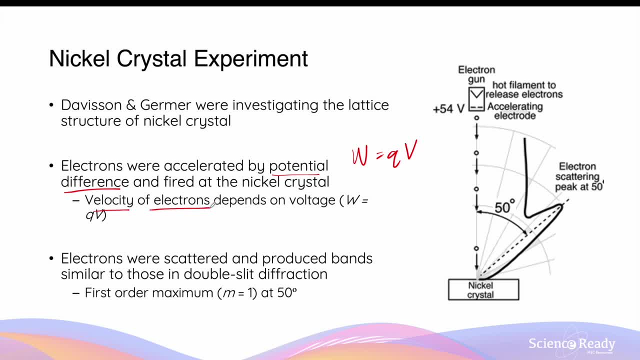 So we can use this to find the velocity of the electrons. In other words, the velocity of the electrons that were fired at the nickel crystal depended on the voltage that was used to accelerate them in the first place. When electrons reached the nickel crystal, they were scattered and they produced band. 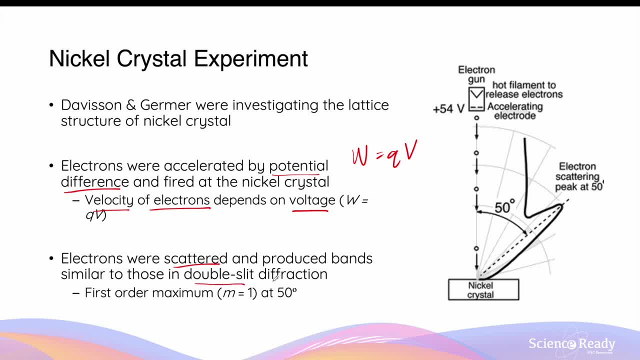 patterns that were similar to those in the double slit diffraction experiment involving lights. Specifically, Davisson and Germann were using electrons to accelerate the nickel crystal. Davisson and Germann observed that there was a first order maximum, that is, mxl1, forming 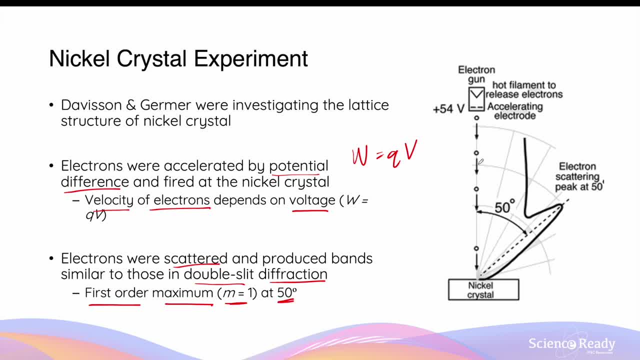 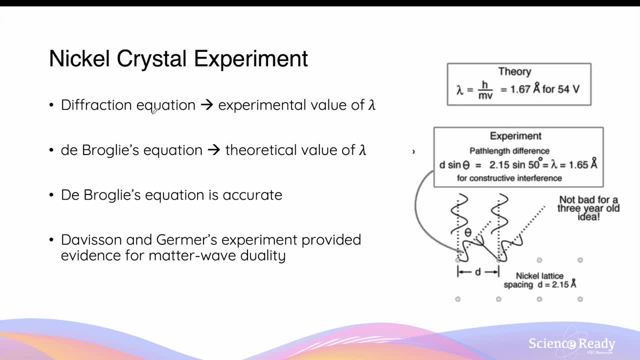 at roughly 50 degrees relative to the midline where the electrons were reaching the nickel crystal. Remember this angle for now, as this will become important later on. Davisson and Germann: after noticing the diffraction pattern, they used the equation for diffraction. 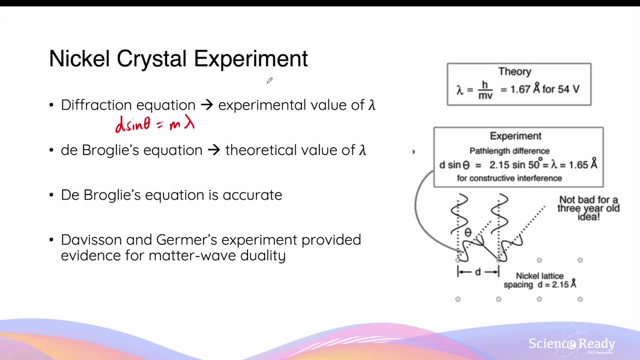 which is d sine theta, equals to m lambda to calculate the experimental value for the wavelength of electrons. When electrons reached the nickel crystal, they underwent diffraction because the distance between the atoms of the nickel was so small that they effectively acted as a small aperture. 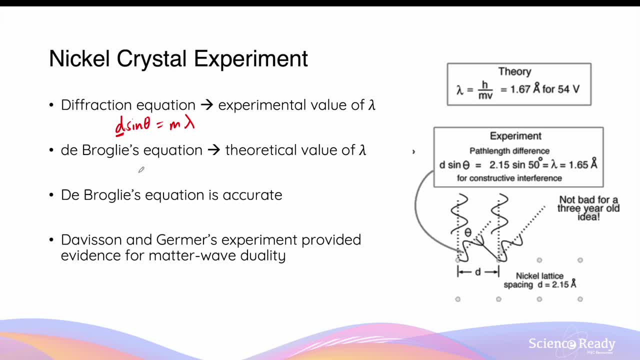 causing diffraction. Therefore, the variable d in this equation is referring to the distance between the atoms of nickel. The variable theta is the angle at which the maximum was formed. In our case, when m, which is the order, was 1, the angle was 50 degrees, which is what 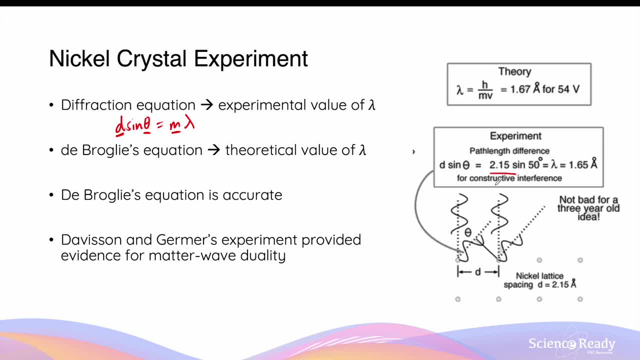 they observed By putting these numbers in distance between the atoms of nickel and 50 degrees, which was the angle at which the first maximum was observed, Davisson and Germann calculated the wavelength of electrons, which was 1.65 Armstrong. 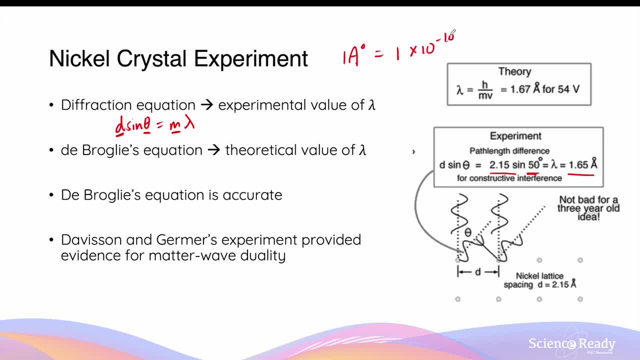 1 Armstrong is equal to 1 times 10 to the power minus 10 meters. so therefore, 1.65 Armstrong is 1.65 times 10 to the power of minus 10 meters. After they calculated the experimental value of lambda, they also used de Broglie's equation. 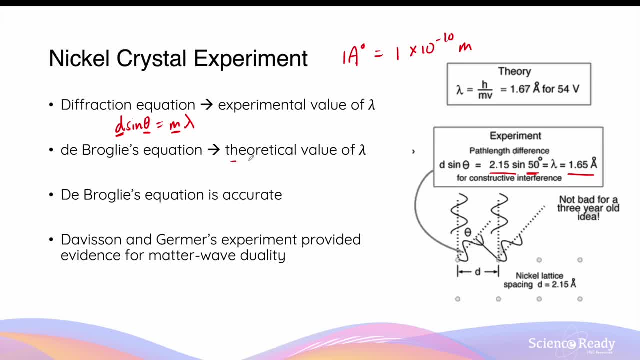 of matter-wave duality to calculate the theoretical value of electrons' wavelength. This is done by using Planck's constant, the mass of the electrons and the velocity of electrons that we discussed earlier. remember the velocity of these electrons was determined by the voltage that was used to accelerate them in the first place. 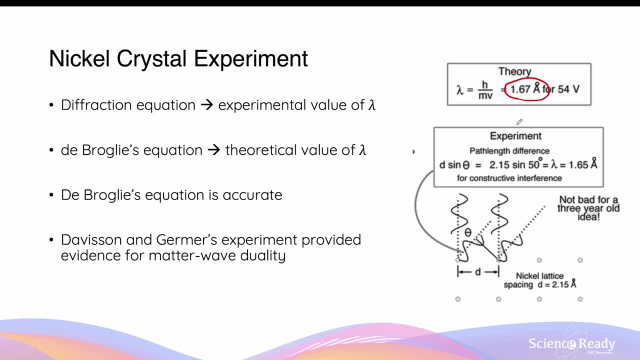 I want you to notice that the theoretical wavelength that was calculated is very similar to the experimental value that the two scientists determined, Because the values are so close. this shows that de Broglie's equation is accurate and, as such, Davisson and Germann's experiment provided evidence for de Broglie's matter-wave.